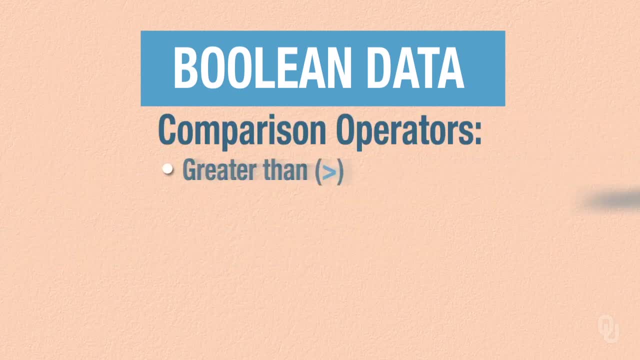 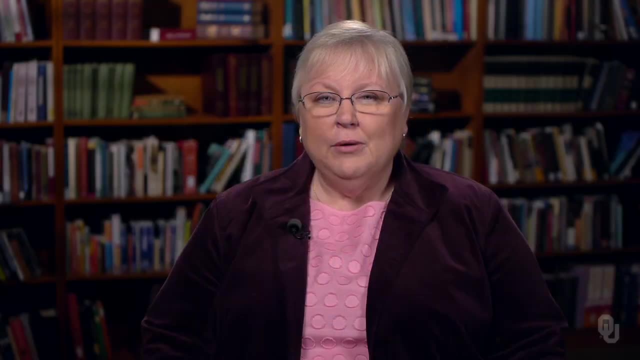 different data type. Boolean data is created mostly by operators like greater than or less than greater than or equal to equal and not equal. Now, equal is a little bit different in Java than it is in math. It's two equal signs put together. 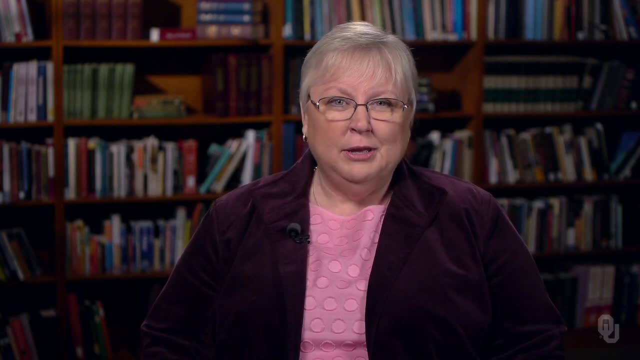 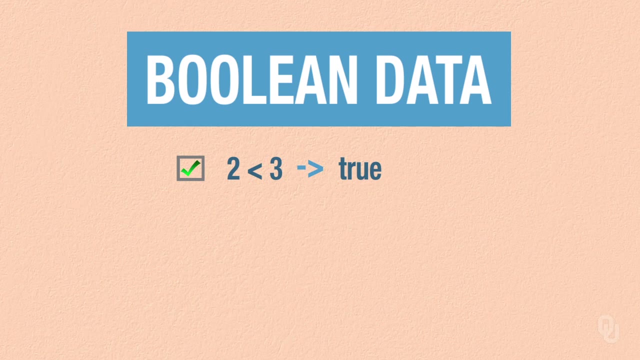 And not equal is an exclamation point followed by an equal sign. So, for example, two less than three has the value true because two in fact is less than three. Five equals equals ten is false because five and ten are not the same value. Five- exclamation point- equals. 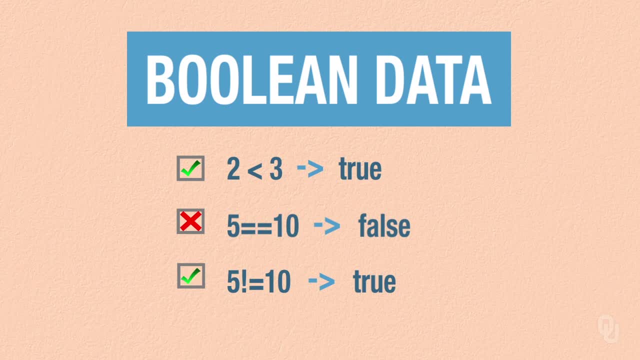 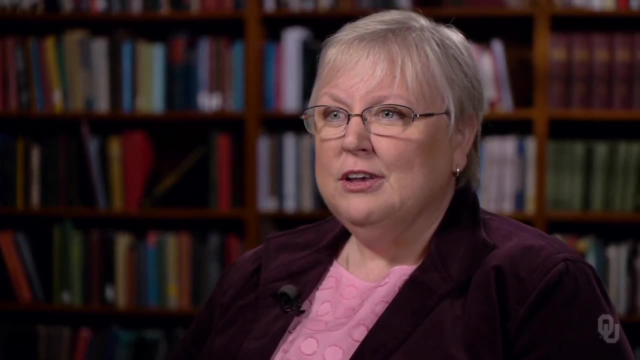 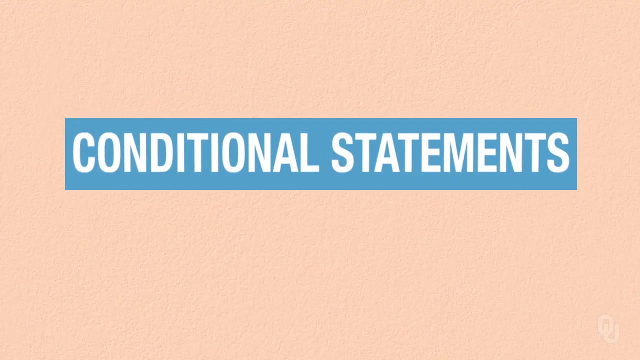 ten, however, is true because five and ten aren't the same. Conditional statements are what allows Java to sometimes do one thing and sometimes do something else. Suppose we have an integer variable that stores the number of tweets that somebody has posted, cleverly called tweets. We could write out that value by saying: you have plus, tweets, plus, and then. 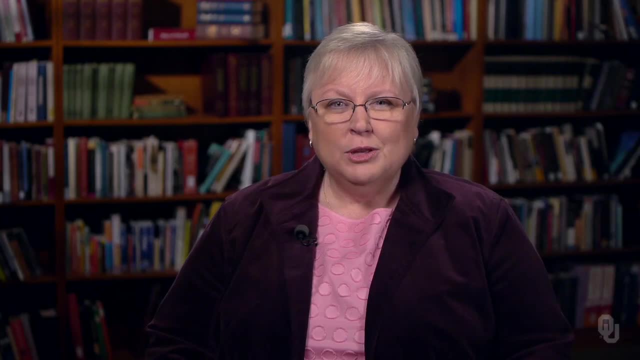 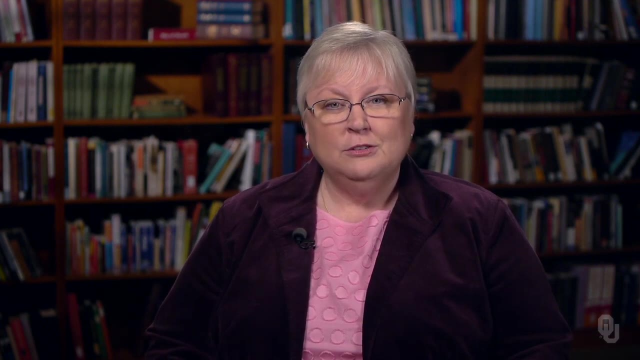 tweets with double quotes where you need them. That isn't really right, or at least it isn't beautiful, because what it should say is: you have one tweet without an s or you have ten tweets with an s. We need to be able to sometimes do one thing and sometimes do something else. 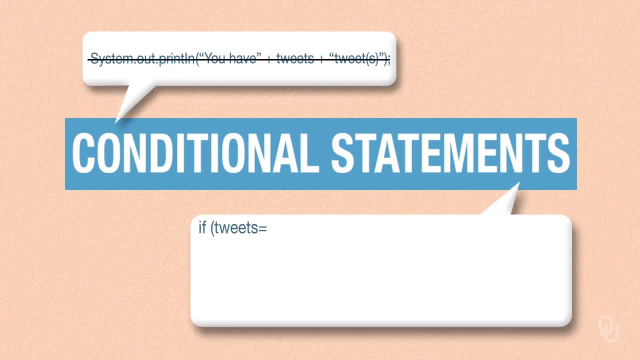 The code that does this looks like this below: If tweets equals equals, one notice, two equals signs, not one system out print line. you have one plus tweets plus tweet. Else system out print line: you have plus tweets plus tweets with an s in it. 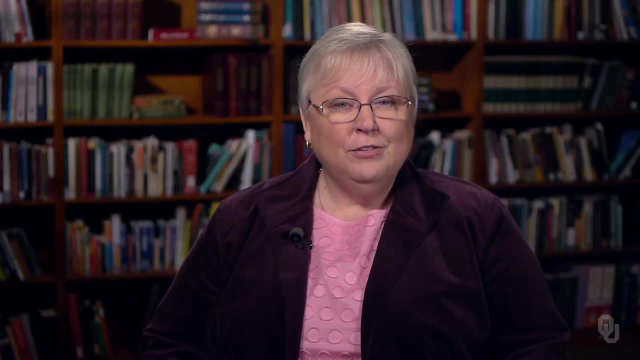 The syntax for this is very simple. The keyword is if. then there's a boolean condition and there's an action that's taken if the condition is true. The else is optional, as are the curly braces if you have only one thing in the statement, like we do in this case. 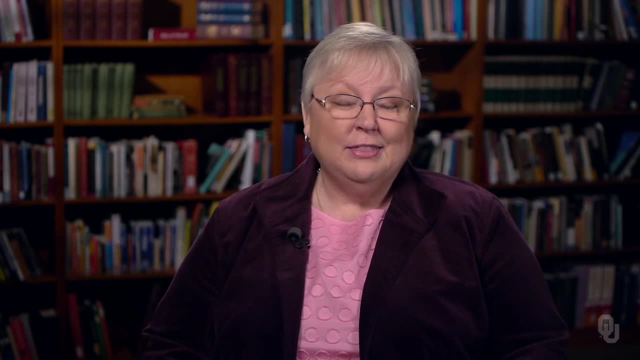 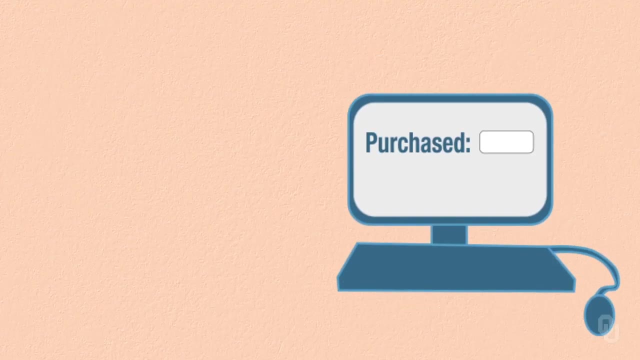 But to tell you the truth, I put the curly braces in most of the time because I think it makes the code easier to read. Let's look at another example. Let's let a user re-enter the number of items they purchased. if they select a negative number To do this, we'll create a scanner Scanner. input is new. 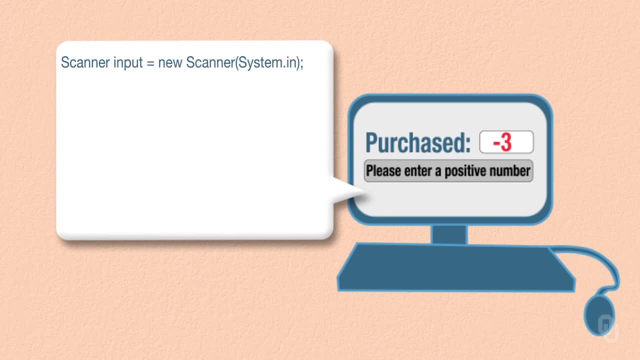 scanner system in. Then we'll create a variable to store the number they purchased, int purchase. We'll say purchase is input, dot next int to let the user enter the number they've purchased. If purchase is less than zero, we'll do system out print line. please enter a positive number. 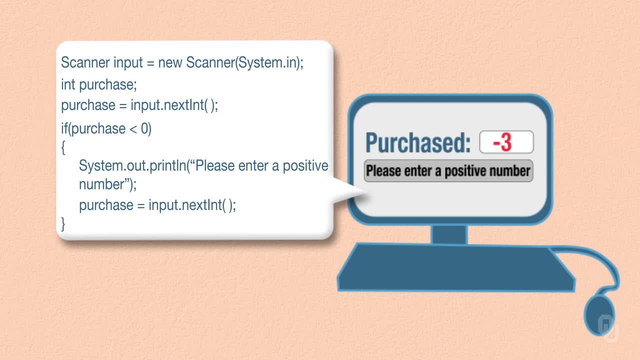 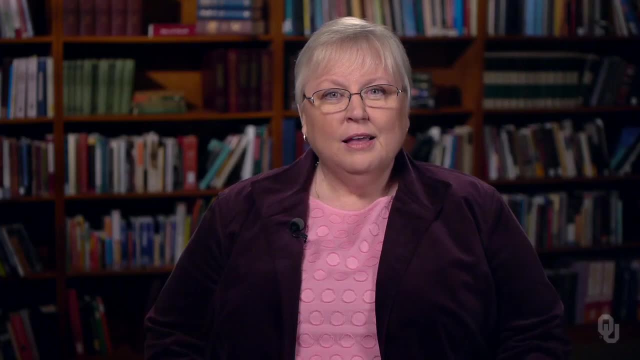 and then purchase equals input dot next int. Notice: this time the curly braces aren't optional, because we have two things that we want to do when the statement is true, not just one. There's a problem, though. Users can make more than one mistake. This code successfully corrects. 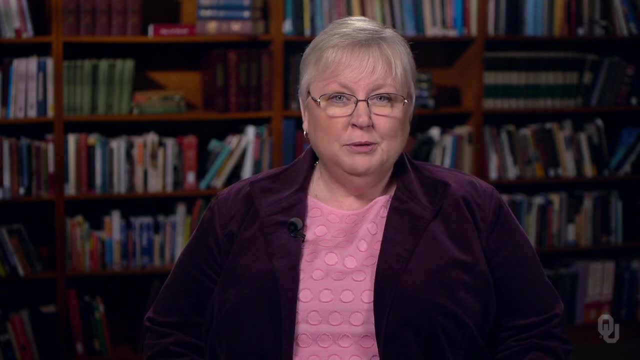 one mistake but then lets the second one slip by. This could be tragic for a vendor, because if a negative order is recorded, it might result in a refund- Definitely not what you want to be doing. And even if you catch this problem later, you're still not helping the customer order correctly, which is very important. 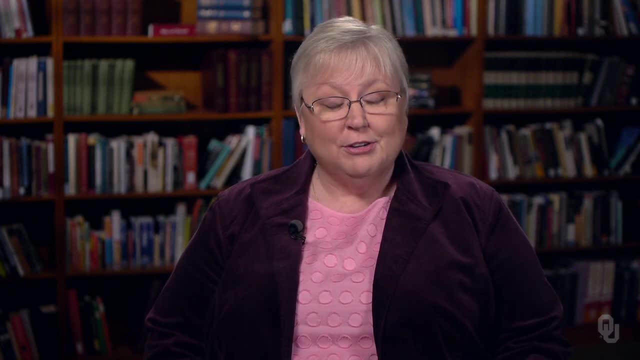 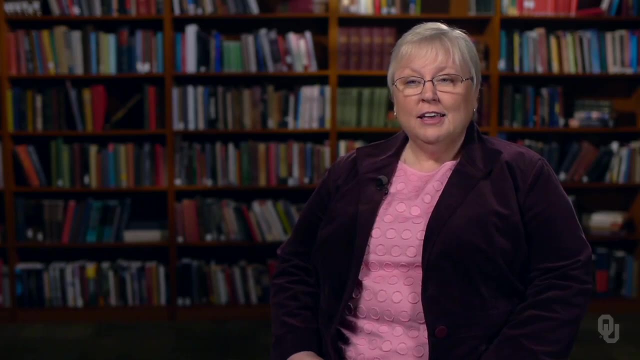 There's a saying in programming that it's hard to make things foolproof because fools are so clever. To fix this, we need to know how to do things more than once. Repetition uses a Boolean condition, just like else does. The code looks like this, while then the 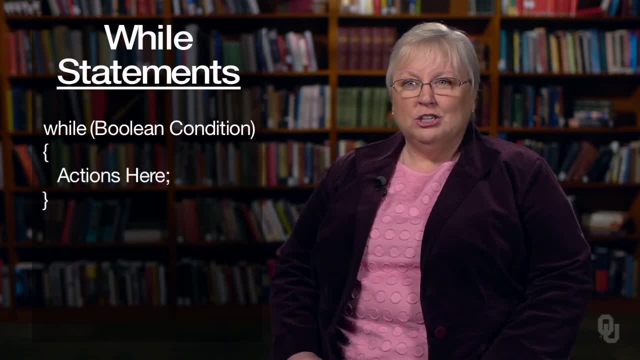 parentheses and then curly braces that surround some actions, Just like if the curly braces are unnecessary, if there's only one statement. but with while loops there's almost never only one statement, so just get used to putting the curly braces in. Here's the while loop. 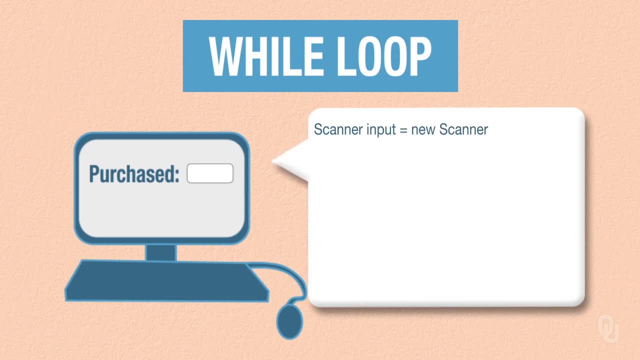 that solves our problem. Scanner input is new scanner system in. Then we need to create a variable to store our purchase, int purchase. We need to get the number of purchases from the user- Purchase equals input dot, next int. And now we need a loop that will allow them to enter it repeatedly So while purchase. 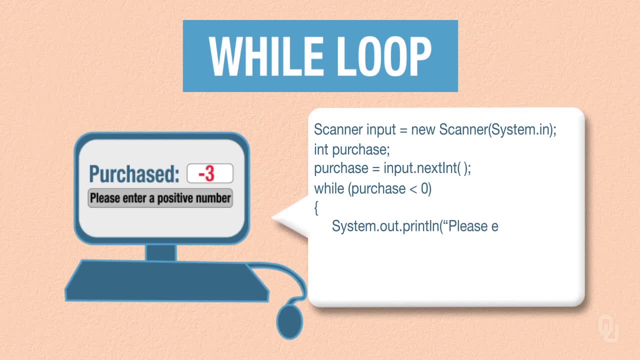 is less than zero. system out print line. please enter a positive number And then purchase equals input dot next int. This loop will run as many times as the user makes mistakes, so we know when the loop is finished. they've made a positive order. 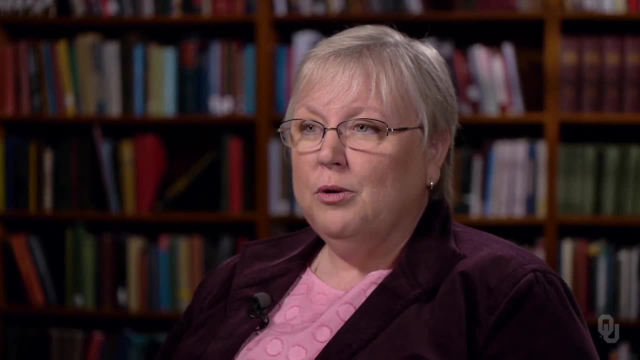 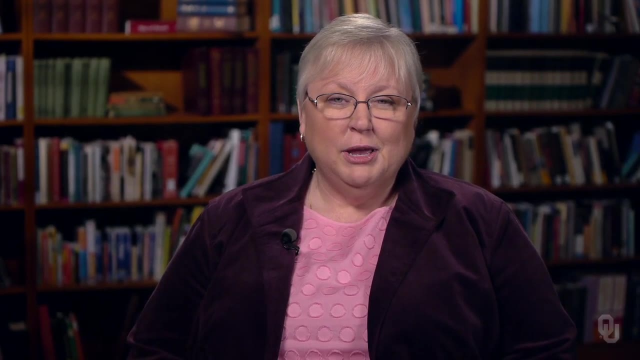 In summary, both if statements and while loops change the order in which program statements are executed, This is called flow of control in programming. Learning to use these statements strategically will make our programs shorter, prettier, easier to read and more powerful.